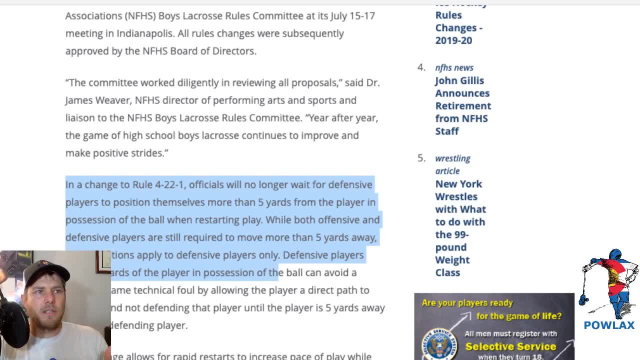 penalty. and this is essentially we're going to be doing the exact same thing as the college rule, and so if a defenseman is within that five yard bubble, if he does not play the player or basically gives that player a complete line to the goal, he won't get an infraction. If he does. 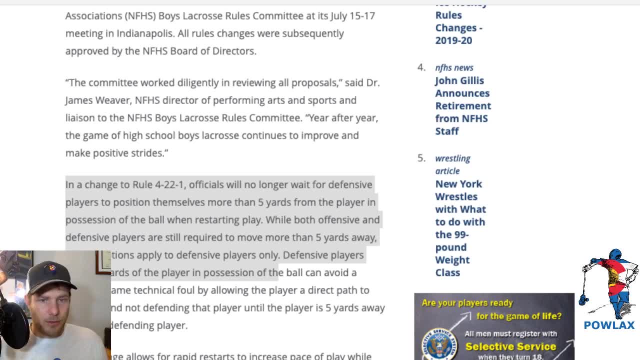 play the player, he will get an infraction. That will be a 30 second penalty. Now this also works from the offensive end. You can't have two offensive players standing with as the ball is being restarted, because it will. you could basically do hidden ball tricks. Essentially, players have to know where the ball is to start a play, and 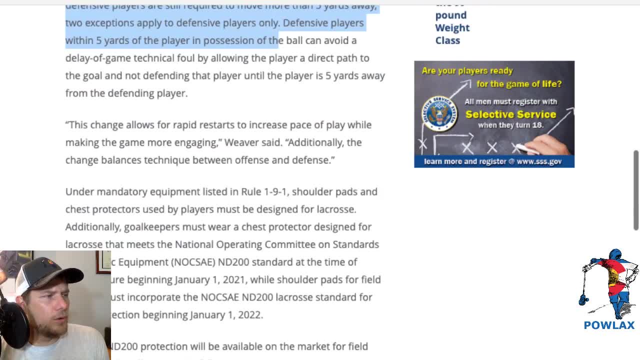 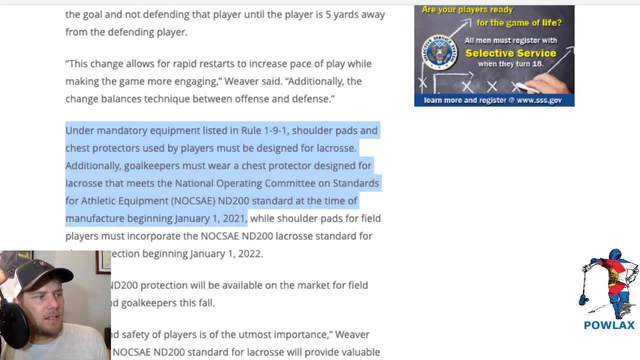 that's essentially the rule. So the next rule that we're going to go over is basically a mandatory equipment rule, Essentially with a new standard, the ND 200 standard, where now everyone's going to have to have lacrosse specific pads. I know a ton of kids who wear hockey pads. This one is going to come into effect in the 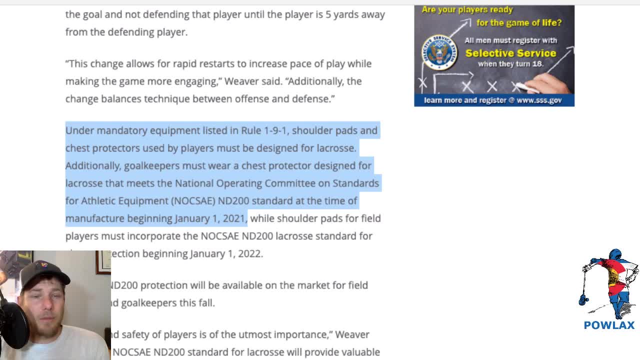 January of 2021 and then chest protectors will be mandated in 2022, and I get it, but I still don't think that anyone's going to not play strictly because they don't have the right kind of shoulder pads. I don't think refs check. 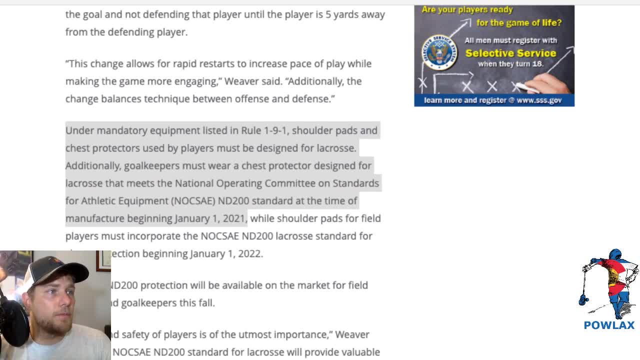 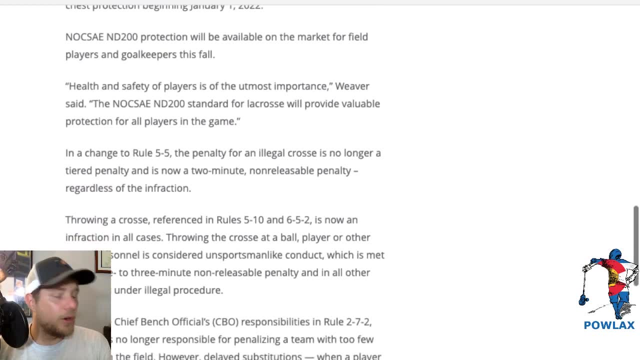 All that much. Now let's see Next one. We've got the health and safety. Okay, Nope, not that. So next one: any violation of an illegal cross is now going to be a two minute non-releasable penalty. 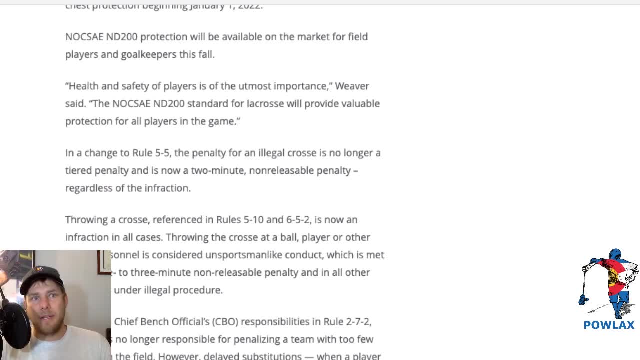 There's no more: one minute for a deep pocket and three minutes for an illegal shape of the stick, essentially, But so it's basically going to bring everything illegal stick wise to one simple rule, which I like a lot. Also, according to um, the us lacrosse magazine, 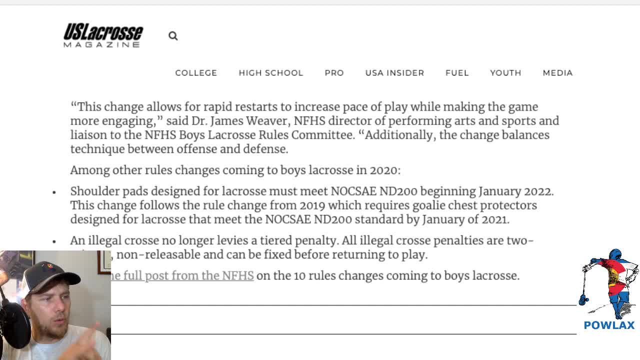 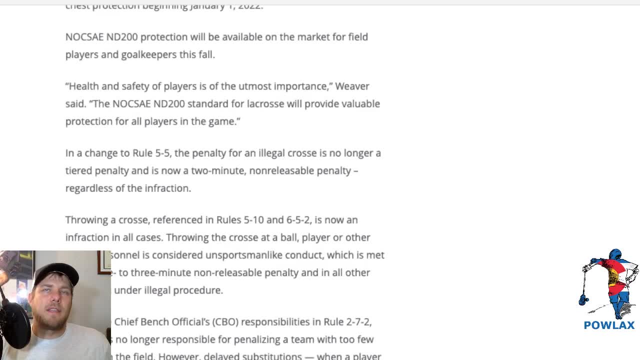 they're saying that you will also be able to alter your stick again and use the same stick, So it won't be the situation back where, basically, the stick would have to sit in the box for the entire game. You're going to have the ability to change it. 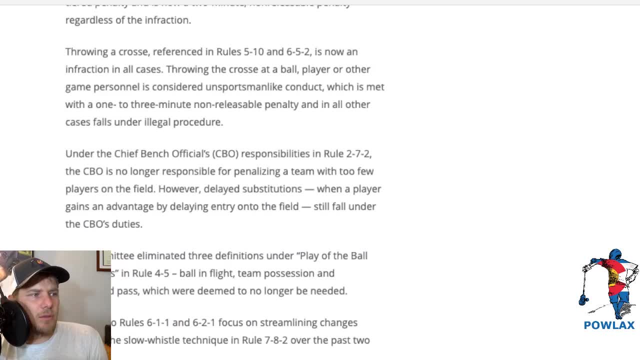 Okay, Next one: the chief bench officials, responsibilities and rule two: seven or two dash seven, dash two, The. basically, they're no longer responsible for penalizing the team with too few players on the field. However delayed substitutions when a player gains an advantage. 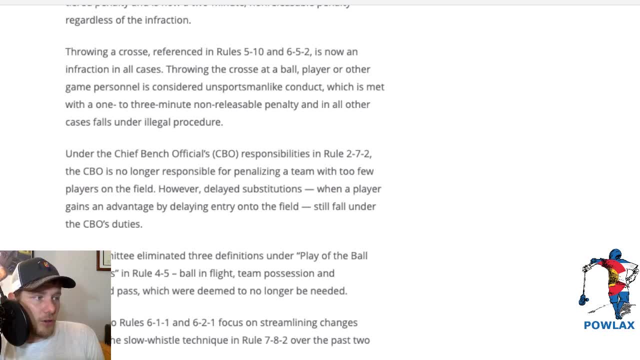 by delaying entry onto the field is still going to fall under the CBOs duties, So I guess he's no longer responsible for penalizing the team with too few players. I don't know if that means there's no longer a penalty for penalizing the team with too few players. 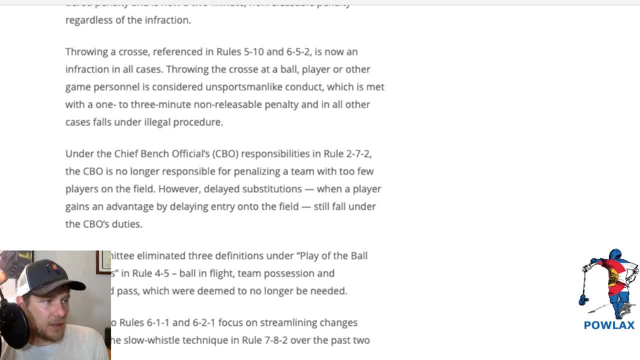 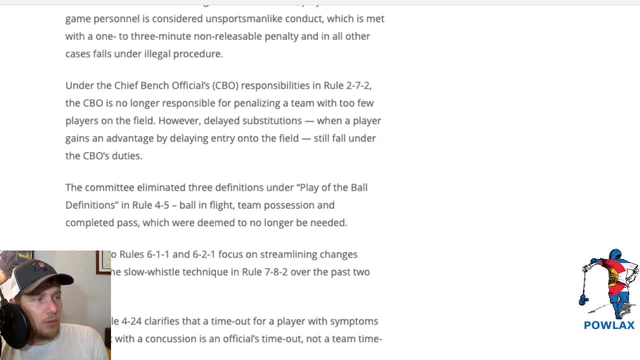 No more penalty for too few players and gaining an advantage, but that's just what it sounds like. So then, they eliminated three definitions of play the ball, which is rule four, dash five, basically ball in flight, team possession and completed pass were deemed no longer needed. 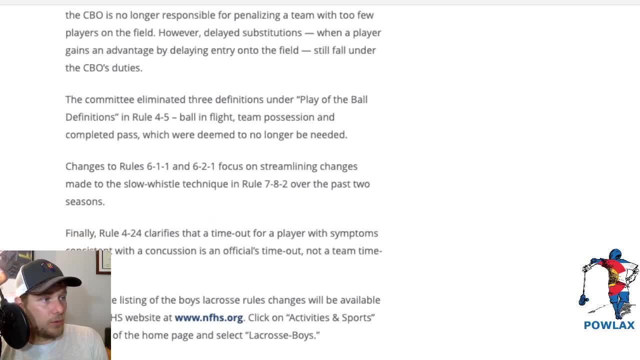 Um, so that's basically just simplification of the rules. Then you have changes to six dash one dash one and six dash two dash one. that focused on streamlining changes made to the slow whistle technique And rule seven dash eight dash two over the past two seasons. I'm pretty sure that this has to do. 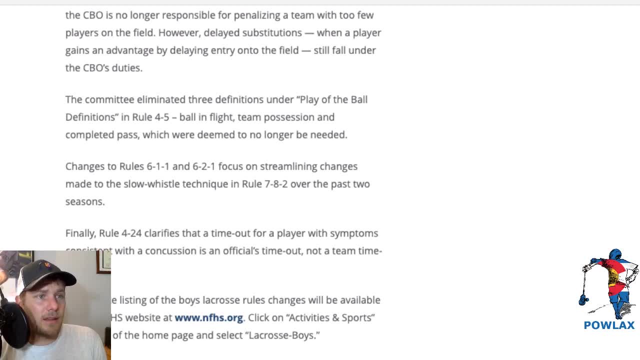 with facing off, but I'm not positive. If anyone can check me on that, that would be appreciated. Um, finally, rule four, dash 24, clarifies that a timeout for a player with symptoms consistent with a concussion is an official's timeout, not a team timeout. That one I like because 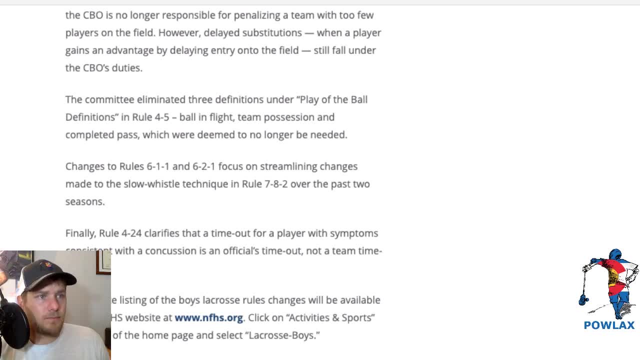 if a kid gets a concussion, it shouldn't penalize either team Um other than a kid. if he hit him in the head, obviously that's going to be a penalty. If you hit a kid head to head, you're going to get a penalty. So that's going to be a penalty. So that's. 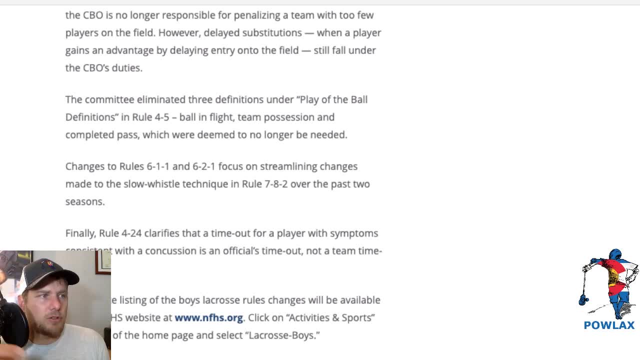 going to be a penalty for the most part. It should be locked in. Also, if you have the ball and duck your head and hit a kid and he gets a concussion, you're also. you should also be penalized. Okay, So now as we're done with this, I want to talk a little more in depth on a couple. 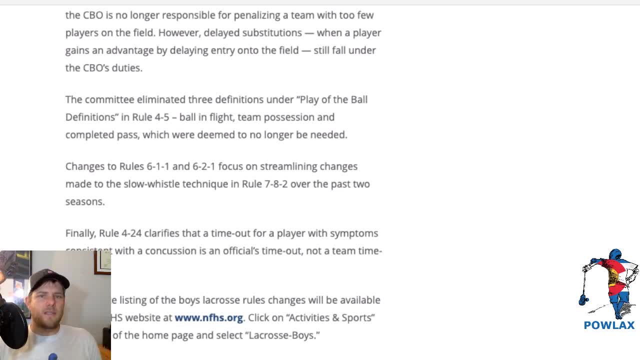 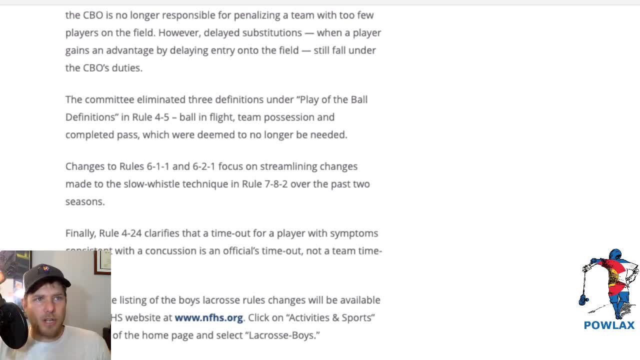 a lot more simple for parents to understand. One of my problems with changing the rules every year is that parents get kind of left behind, because refs and coaches usually tend to work out new rules in the fall. But if parents aren't kind of brought along, they might not kind of. 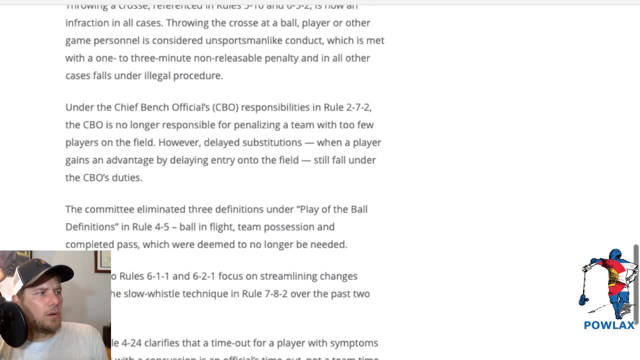 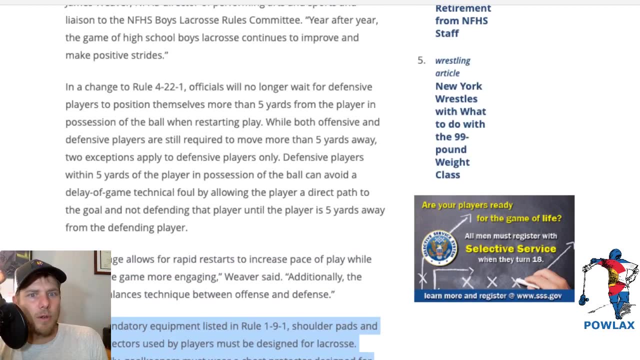 understand Um. so now the next one that I'm really excited about is this: um, basically quick whistle rule. So so many of our players were excited about the illegal stick penalty And they were excited to play by quick whistle rules because they were um, they were watching the 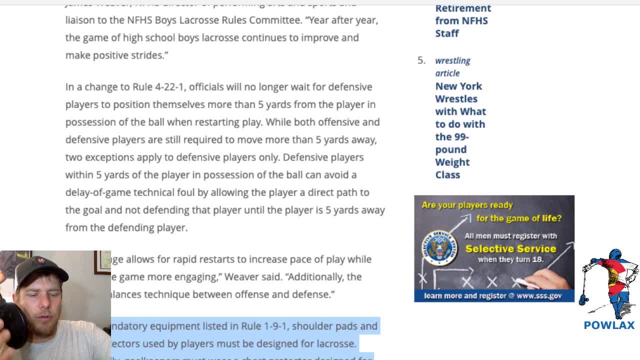 college game, And so they'd pick up the ball, they'd be ready to go, And the ref wouldn't blow the whistle. And it was very frustrating for them because they'd been watching games where that was the case, And so the ref would slow them down. you know high school kids, they'd get all pissy. 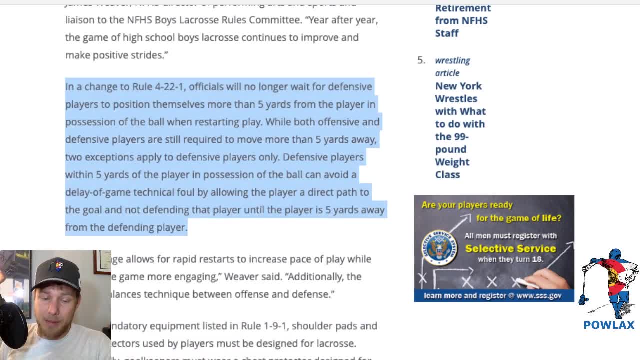 And so now this will be better because it will look like the college game that they're seeing. you know, no dive, no, none of that crap, but at least it'll be a quick game, And so for that we have a little video of exactly what that looks like. So 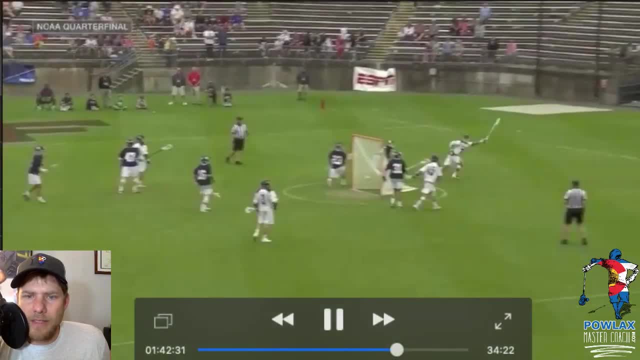 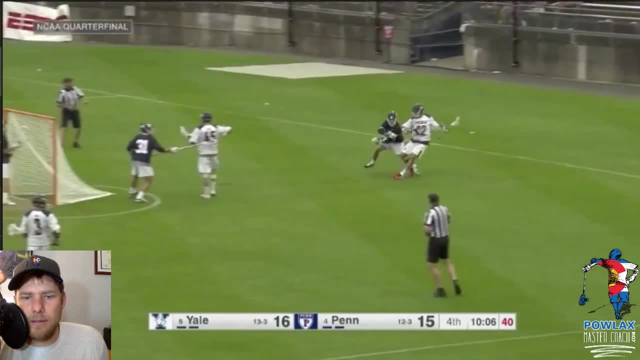 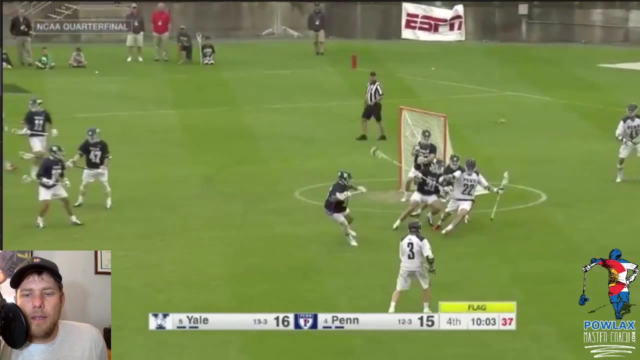 as we play this out. essentially, the ball goes out of bounds on a shot. The ball is picked up, Penn brings it in on the field and notice that the Yale player, the L defenseman, was playing that player And so he would get a penalty here. Now you see the ref throw the flag, the call. 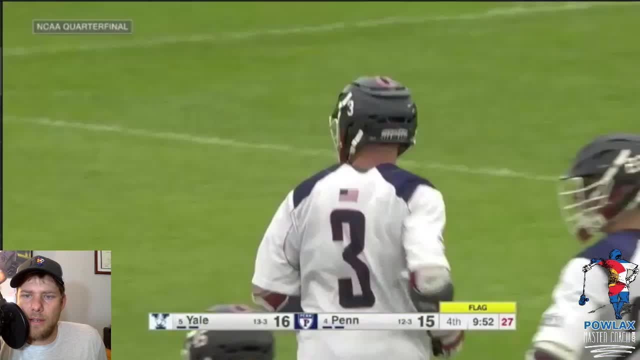 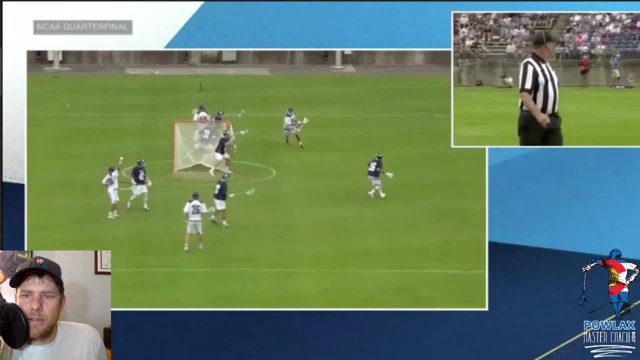 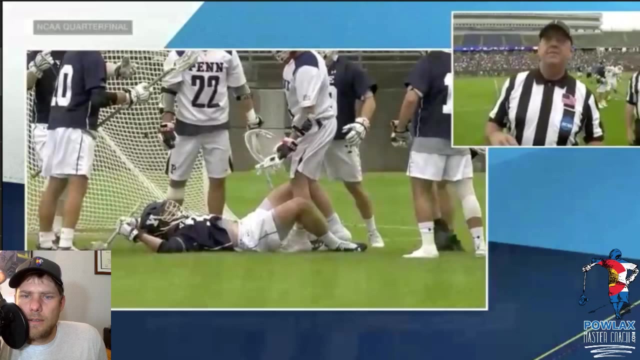 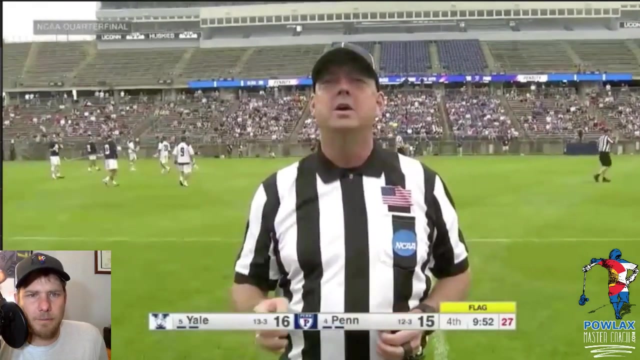 let's see what motion he makes. He makes say: let's see, I want to say it's a legal procedure, It should be a legal procedure. Let's see what he does: Technical foul, legal procedure. Okay, So he was basically too close to him as he came in out of. 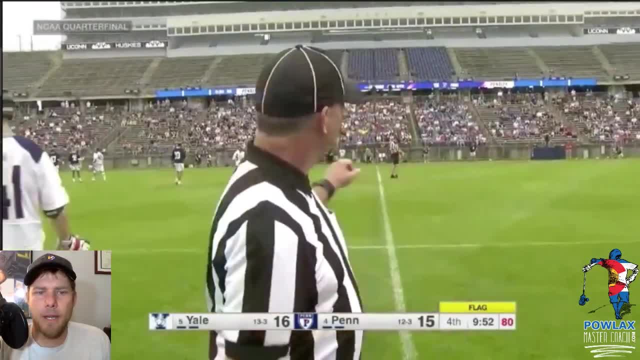 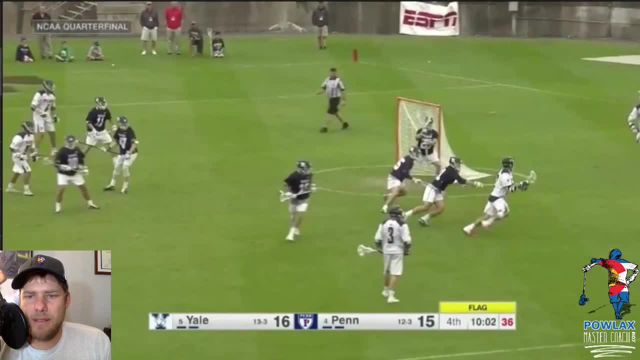 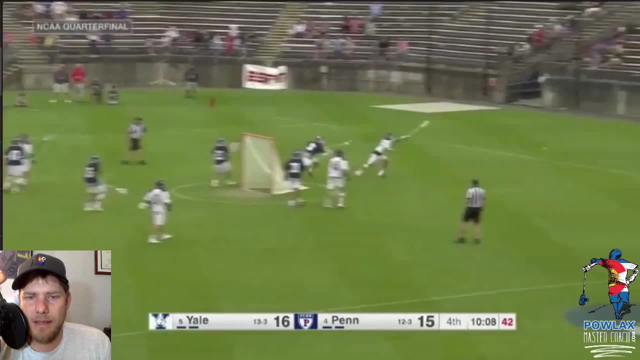 bounds, Excuse me. Okay, So that's what the rule will look like. So now to clarify on this rule: in this event, when he is coming off the end line and they're close together, it makes sense that the defenseman is responsible. Now, if the defenseman stays behind, 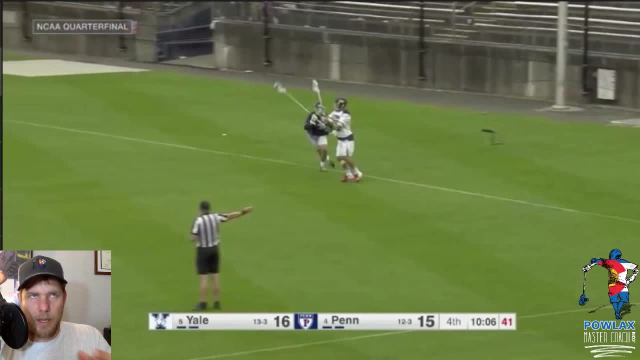 him. so right here the whistle blows, he's going into play. If the defenseman does not play him and allows him to move ahead until the Penn player has passed five yards, that is not a penalty. So essentially, defensemen who get caught in that position need to basically just 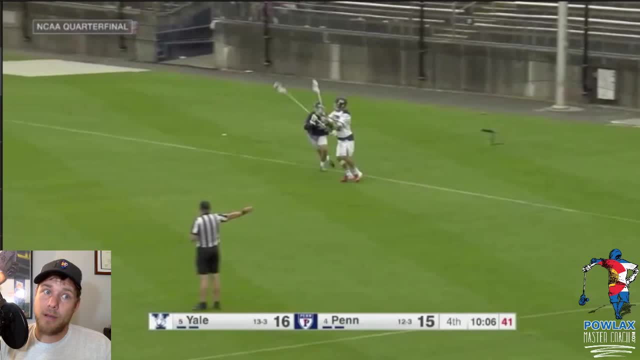 I don't know if you can run the five yards with him or you have to kind of wait there, but basically I'm pretty sure you just can't impede him as he is playing within those five yards. It seems pretty simple. It seems pretty, I mean it's. it makes sense. but so that's the. 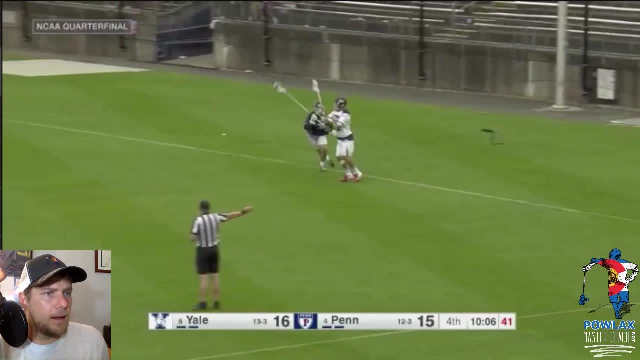 big rule that's kind of coming in. Let's see Now. I don't believe there's any other big rule things that I mean- the shoulder pads ones I get, but it seems to be like the worst time for that kind of rule, with the PLL now doing. 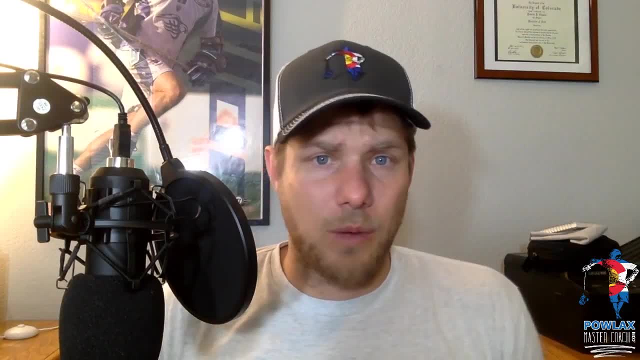 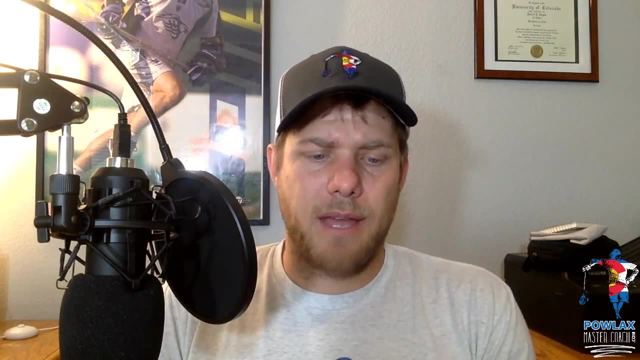 So the PLL is now having players that don't even really wear pads, And so we're going to mandate that high school players have to wear shoulder pads that meet a specific standard. So that's a specific specification, which means every single player is going to have to buy brand new shoulder. 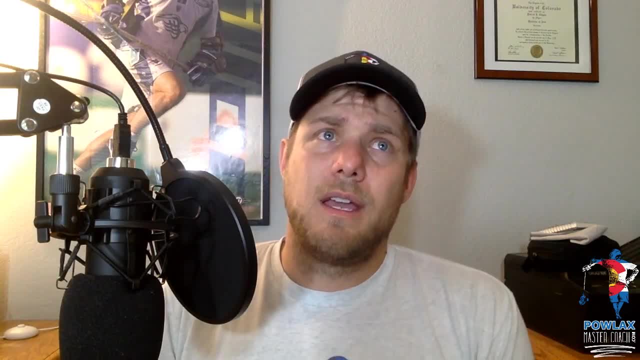 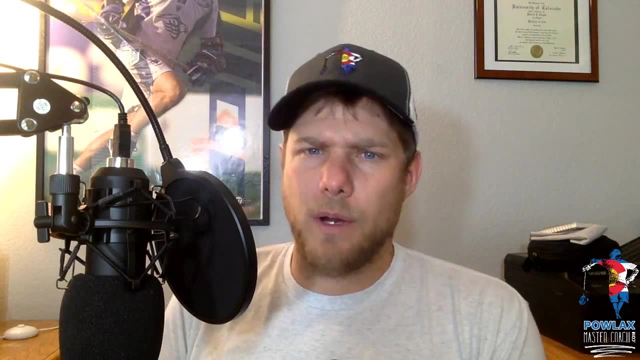 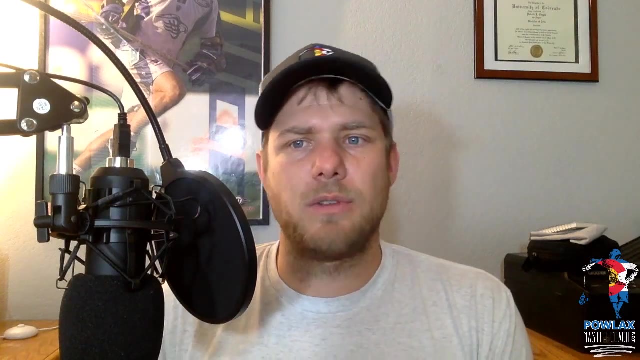 pads in 2021. Yet when the rule is announced, no players in the PLL are actually wearing shoulder pads. I don't know It. just I get the idea of protecting the kids on another level. Anytime I played in high school, it was very small shoulder pads. I hated pads And I mean it was kind of. 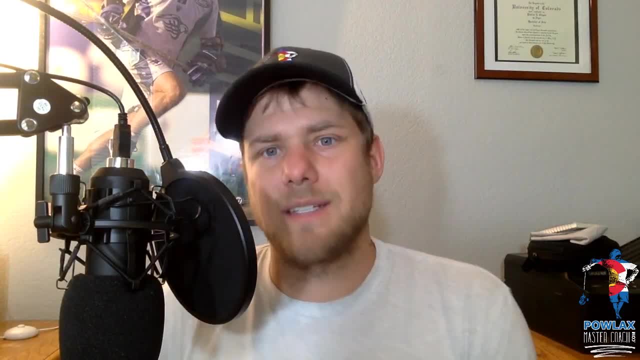 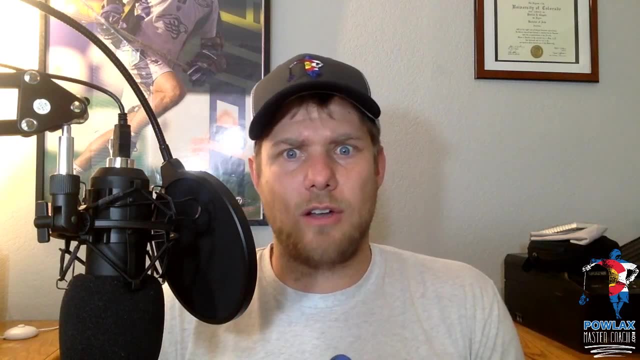 weird because back then I used to think I was cool because I didn't have the shoulder pads. But now I see kids who don't have bicep pads, who can't take a cross check all game And yet, and then they end up being bad in the fourth quarter because you know they've been beaten on the whole time. 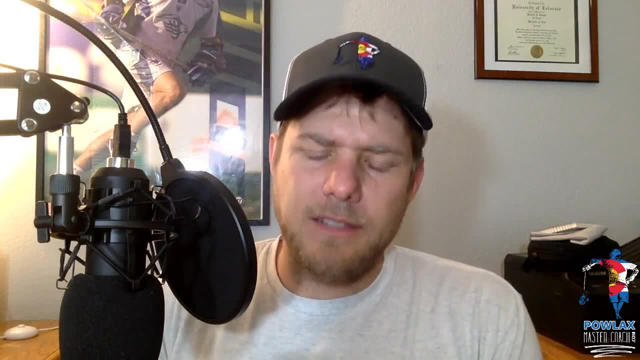 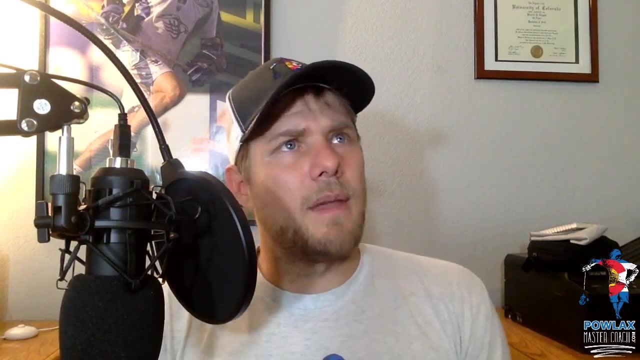 and they could have padded up, but they don't. I don't know. It's an interesting thing with the rules. It seems almost like a money grab for Noxie for me, but that kind of just is what it is, Anything else. Let's see. What are the other? The other one is just the stick penalty. I think that